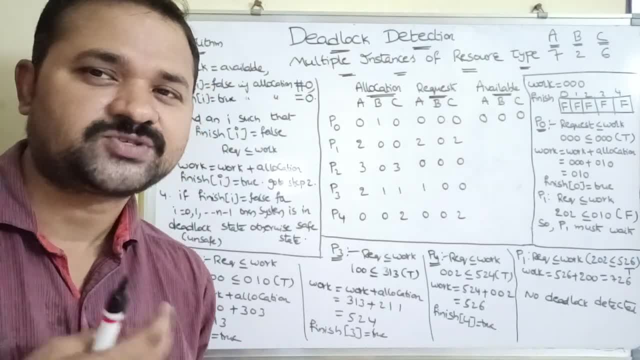 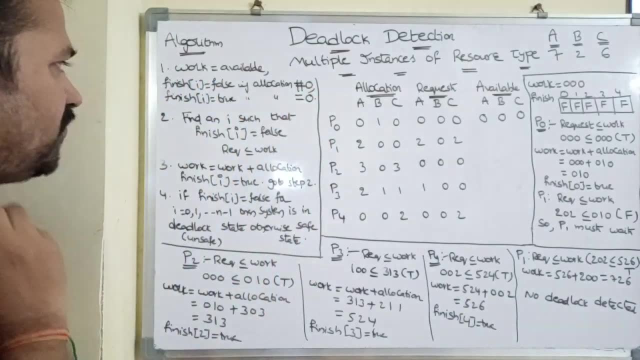 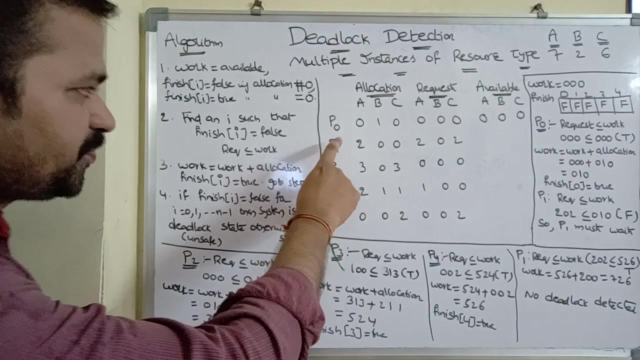 every process will get some allocated resources, So allocation value is always not equal to 0, so if the allocation is not equal to 0, then finish of i is equal to false. so what is i here? so i means the process number from 0 to n minus 1. so for the first process i value 0, for the next: 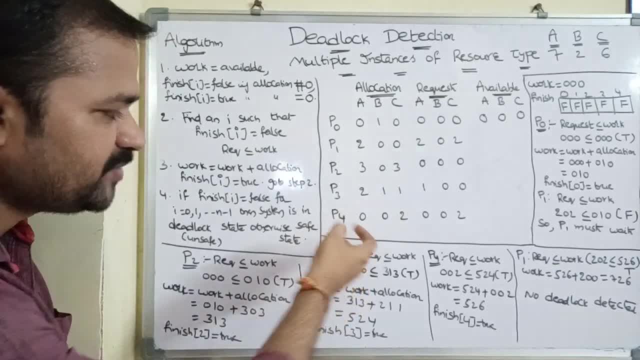 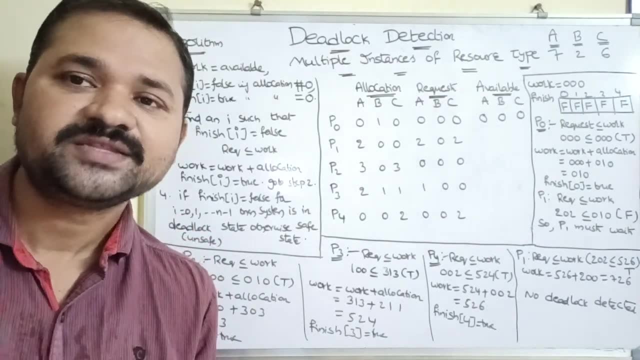 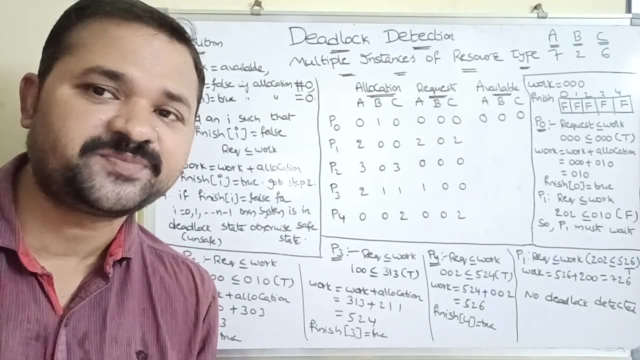 process i value 1, whereas for the last process i value is n minus 1. okay, so if finish of i is, if finish of that process is 0 false, then we can say that the process execution is not completed. let finish of 2 is equal to false, so it specifies that process 2 execution is not completed. 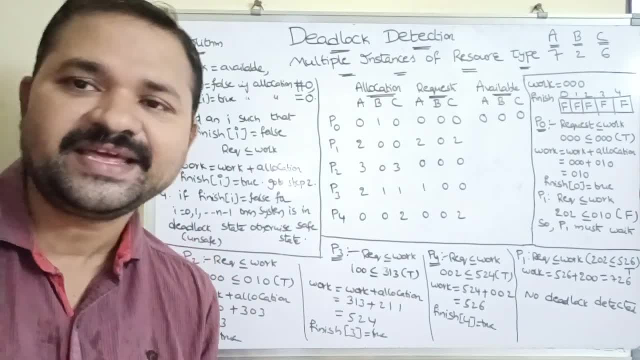 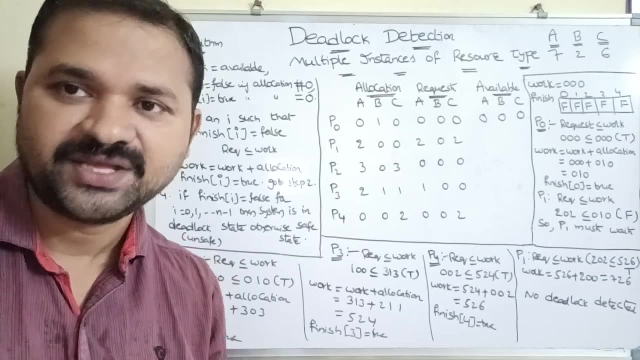 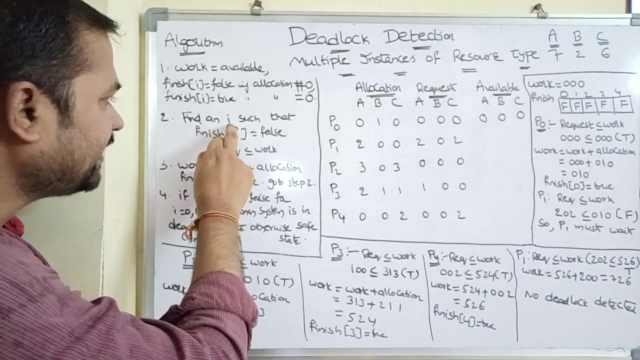 whereas if finish of i is equal to true, then we can say that that process execution is completed. so false means that process execution not completed, whereas true means that process execution is completed. okay, next, what is the second step? find yan i such that. so here i means. 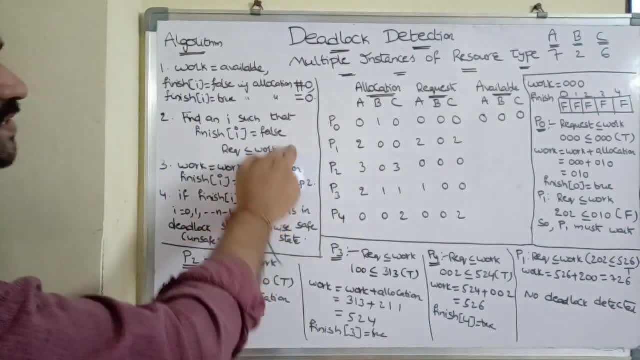 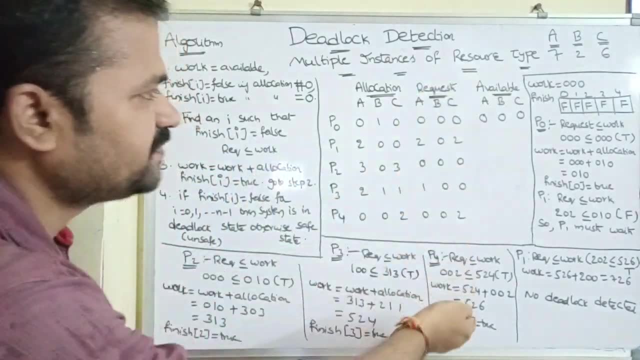 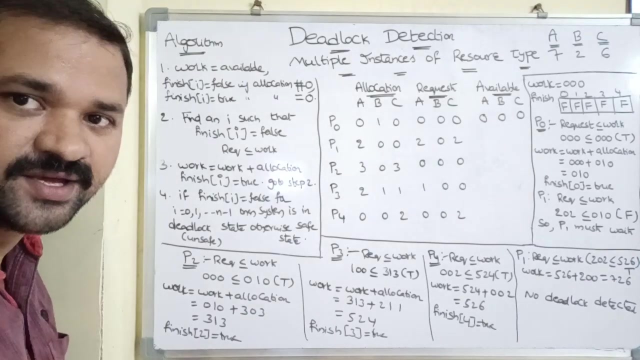 the process number. finish of i is equal to false. you initially finish of i value is false. only request is less than or equal to work. here this is nothing but request and this is nothing but work if request is less than or equal to work. so what means available resources? then operating system can allocates available number of resources to the 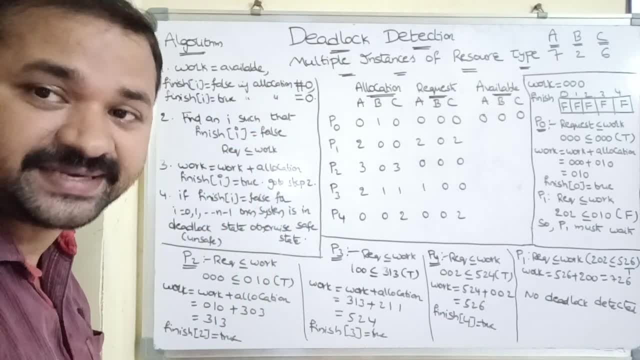 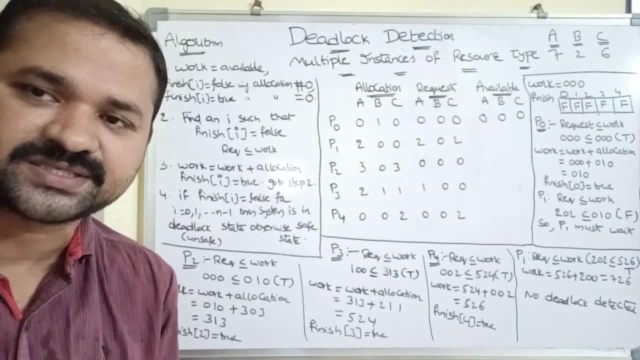 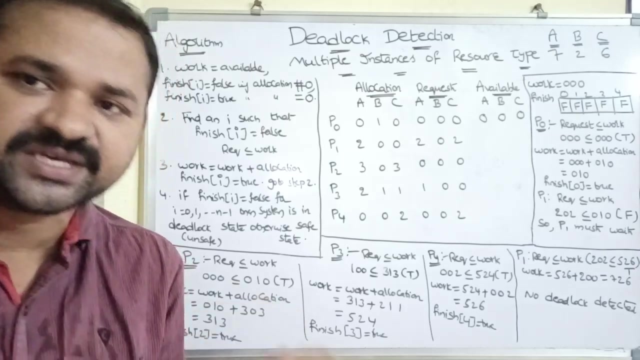 corresponding process so that process can complete its execution. so once the process execution is completed, then the process will be moved from main memory to the hot disk so we can remove allocated resources from that process and we add allocated resources of that process to the available resources. why? because no longer that process is not needed now. so that 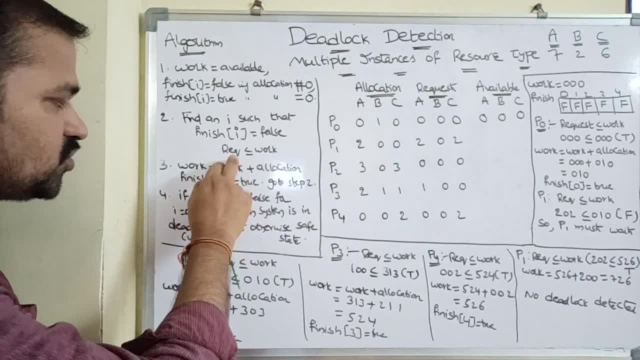 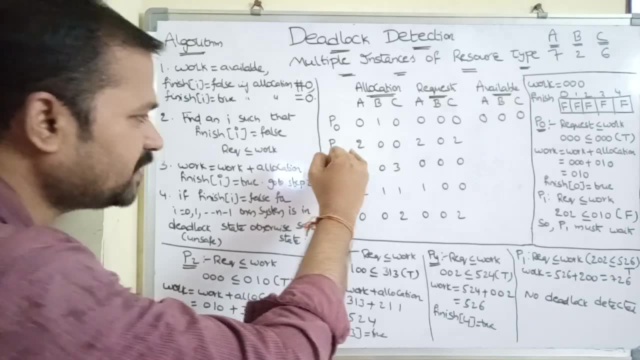 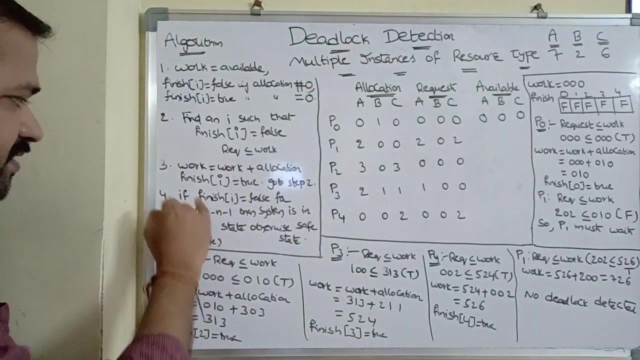 is step 3. work is equal to work plus allocation. so whenever request is less than or equal to work, then we can complete this process execution. so operating system allocates operating system yards allocated resources of that process to the work next to finish of i is equal to. 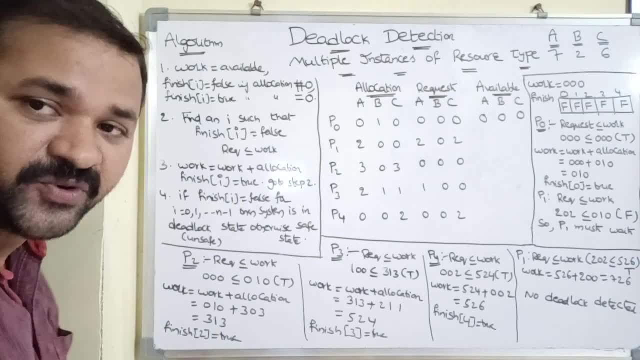 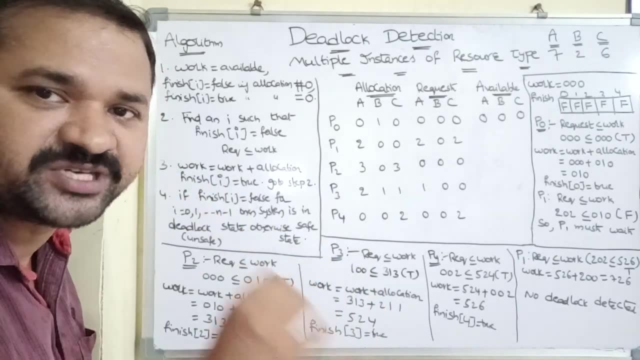 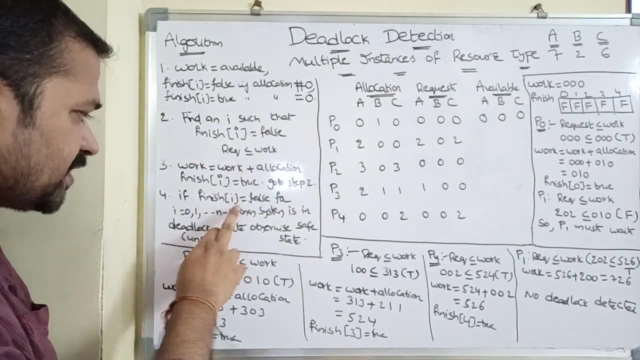 true, why? because this process execution is over. if the process execution is over, then we have to mark finish of that process. yes, true, it specifies that that process execution is completed. next to go to step two. so likewise, we have to search for all the processes. next, what is the last step, if 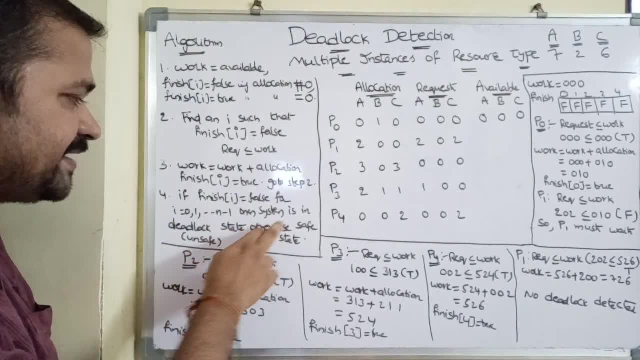 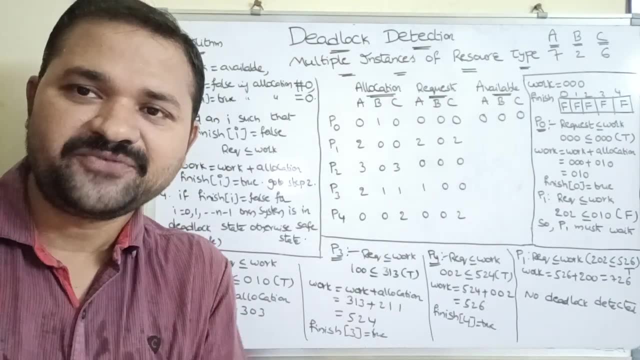 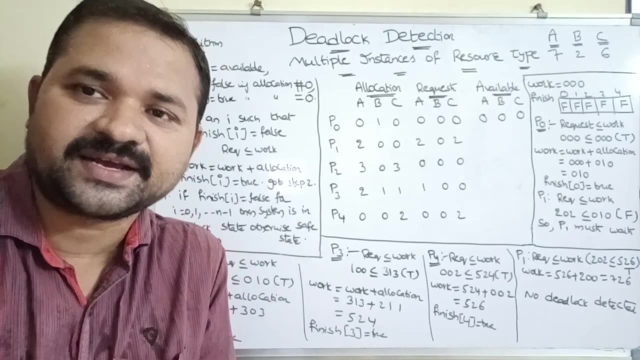 finish of i is equal to false, for i is equal to 0 to n minus 1, then the system is in unsafe state. that is nothing but deadlock. so already we have seen what is false, what is true. if finish of i is false for some processes or for all the processes, then we can say that the corresponding 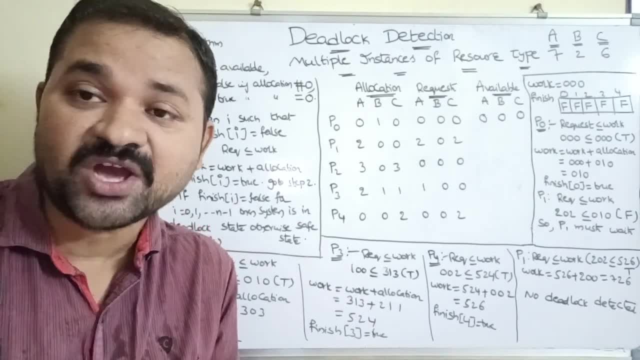 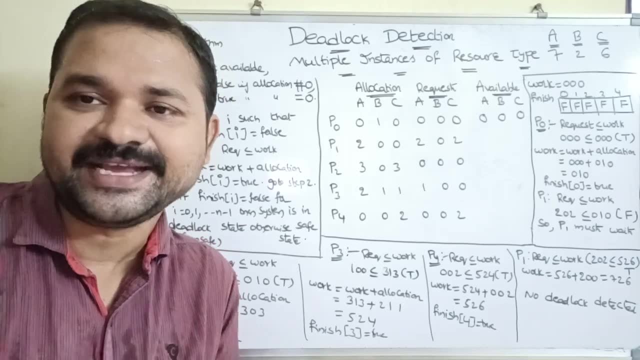 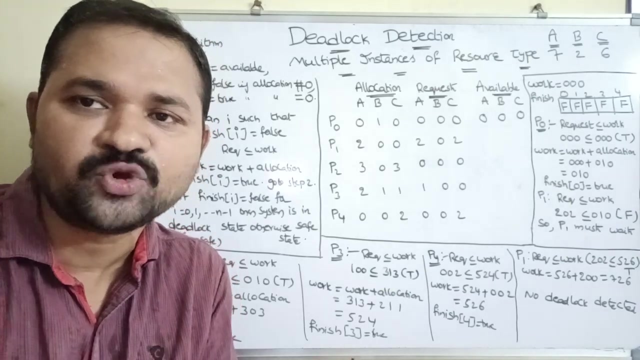 system is suffering with deadlock, whereas if finish of i is true for all the processes, then we can say that there is no deadlock. if there is no deadlock, then it is known as safe state or safe sequence. safe sequence specifies the order in which the processes are to be executed. 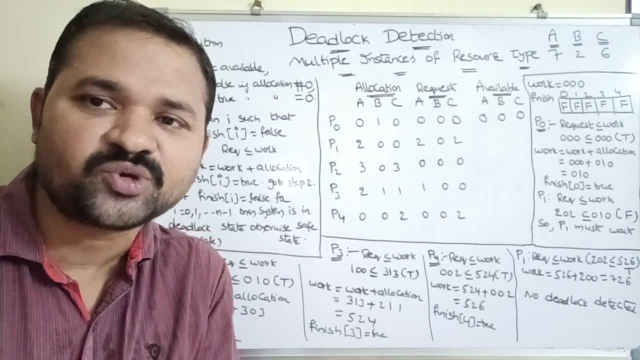 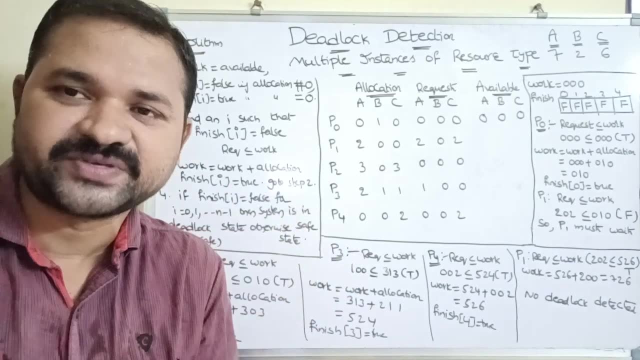 so the order in which operating system allocates resources to the processes. suppose, suppose catalog. for example, if the finish of i is false for few processes or some process or all the processes, then those processes are suffering with deadlock, so we can say that it is in deadlock state. 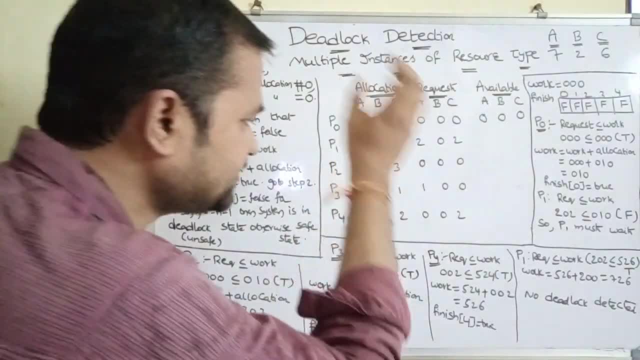 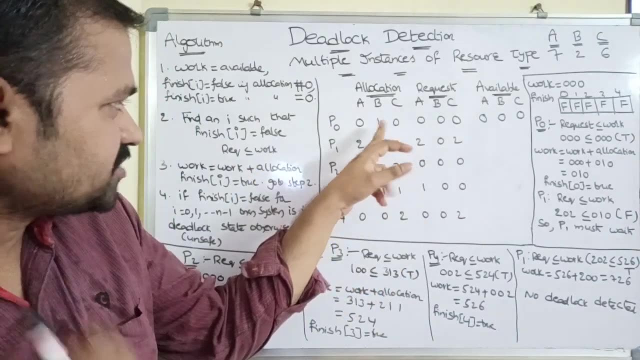 that is nothing but unsafe state. oh, now let us solve this example by taking this algorithm. here we have five processes, from pinor to the p4. so at this moment, so these are the allocated resources, so zero instances of here are allocated. one instance of resource type p is allocated zero. 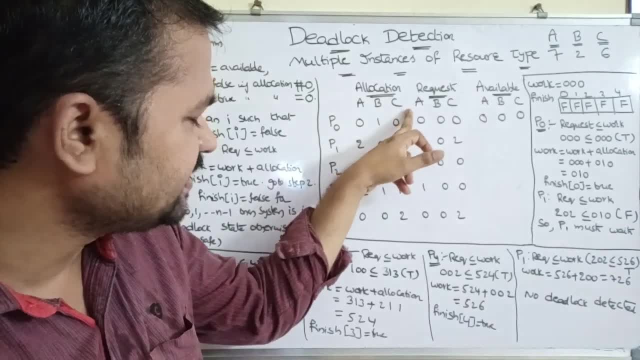 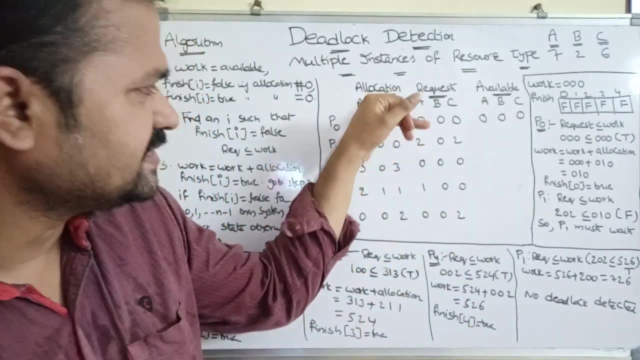 instances of 2 are allocated. so these are the resources. we need to kind of come up with something. zero instance of resource type C is allocated like that: Let A is printer, B is scanner, C is some hard disk. So there is no printer, one hard disk is attached. there is no scanner like that. 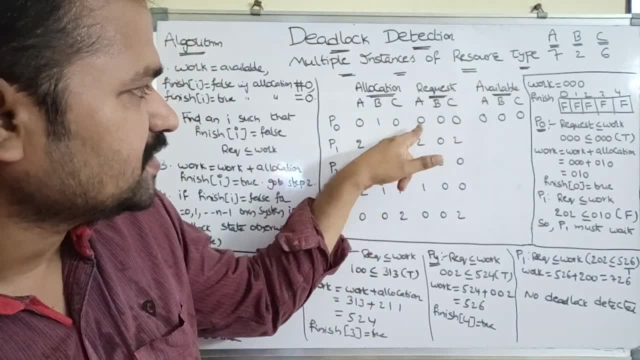 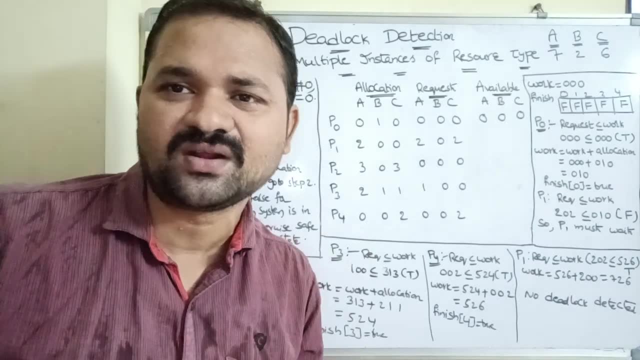 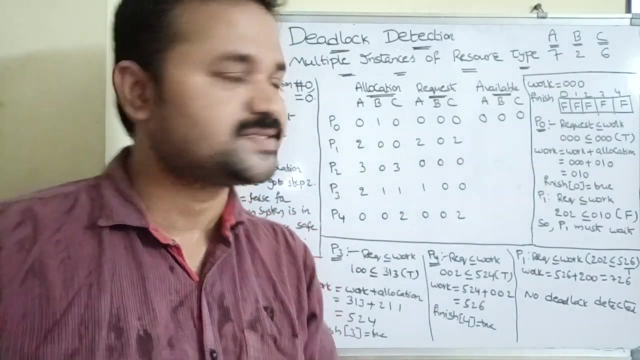 Here. what is P0 request? P0 is requesting for zero instances of A, zero instances of B, zero instances of C. So that means P0 is not requesting for hard disk printer and scanner like that Next year. initially, the available number of resources in the system are 7 to 6.. 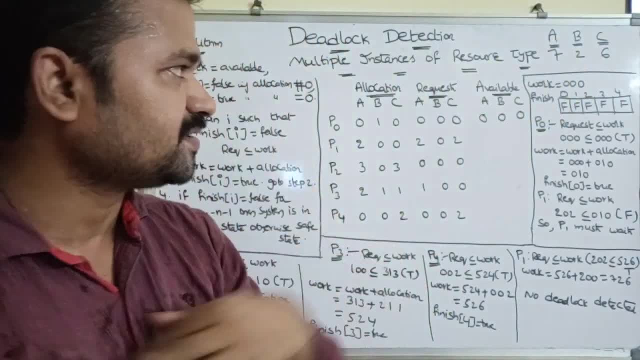 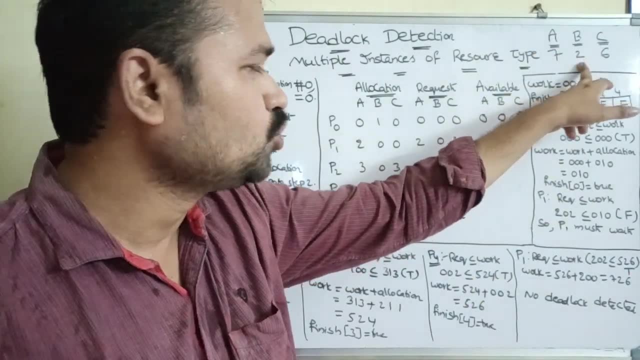 Let: A is printer, B is hard disk, C is scanner. So that means 7 instances are attached to the computer, 7 printers are attached to the computer, 2 hard disks are attached to the computer, 6 scanners are attached to the computer, like that. 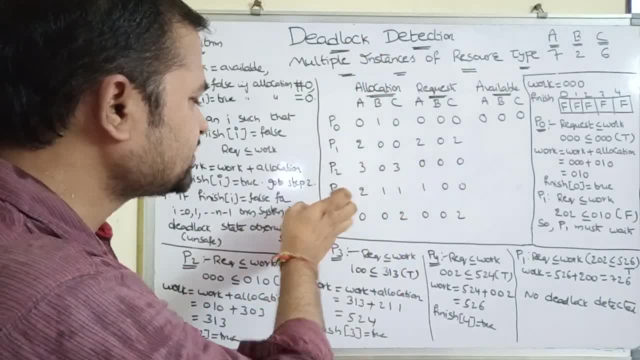 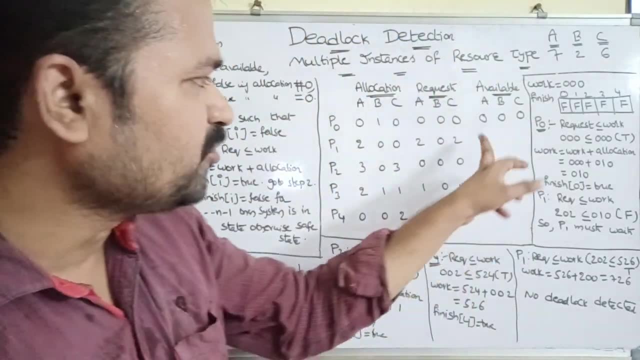 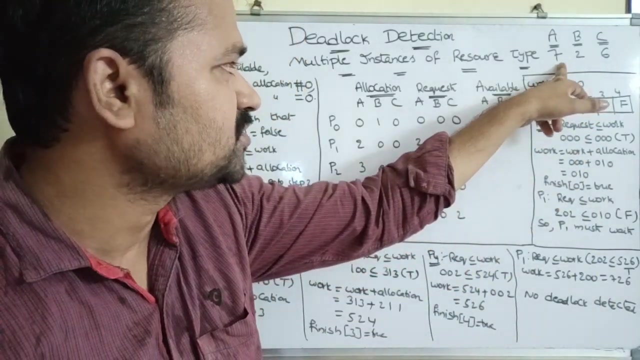 So at a particular time. so these are the allocated resources for these processes, and this is nothing but the request, The demand of the process. Then after that we have to calculate the available resources after performing the allocation resources. So for resource type A, the available resources are 7, but out of 7,. so 2 plus 3 plus 2 means 7.. 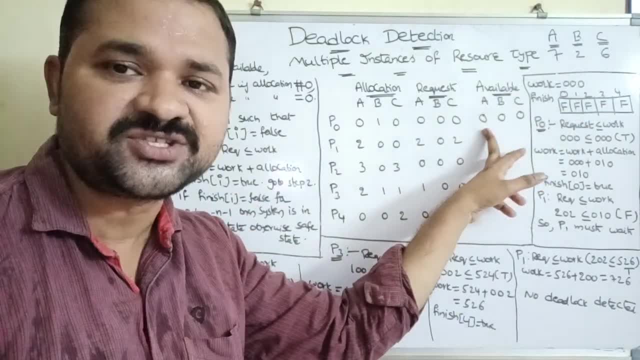 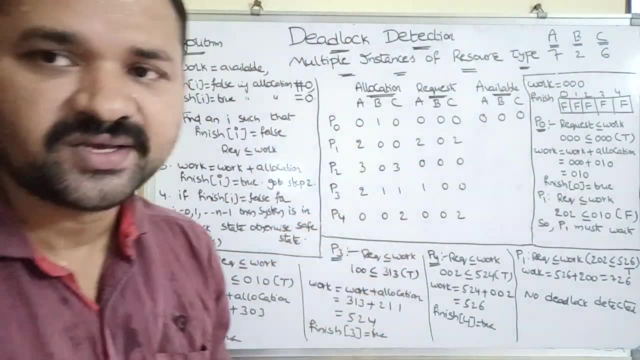 So 7 resources are allocated. So 7 minus 7 means 0.. If you take resource type B, actually we have 2 resources. Out of 2 resources, 2 are allocated. So 2 minus 2 means 0.. 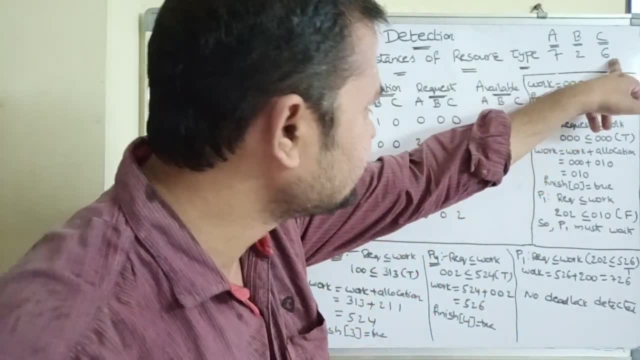 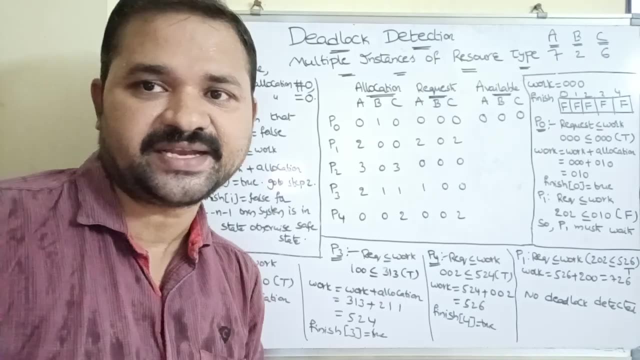 So resource type B means 0.. Next, if you take C, actually we have 6 resources Out of 6, 3 plus 1, 4, 4 plus 2 means 6.. 6 resources are allocated. 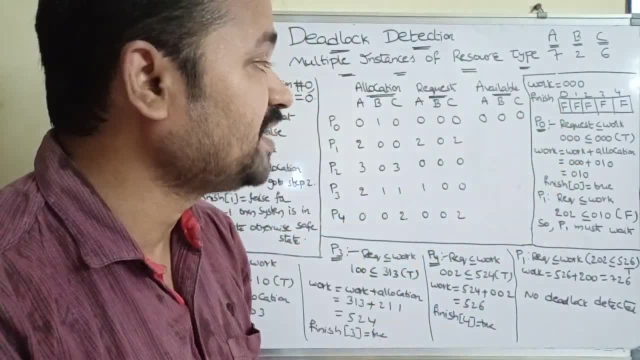 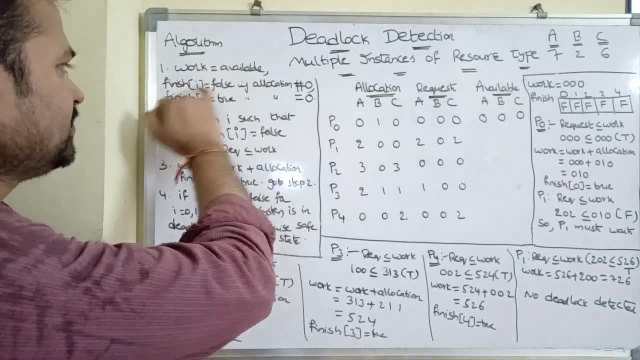 So for resource type C also, the number of available resources are 0.. Now let us solve this problem by taking this example. The first statement is: work is equal to available. The next statement is: finish of I is equal to false. 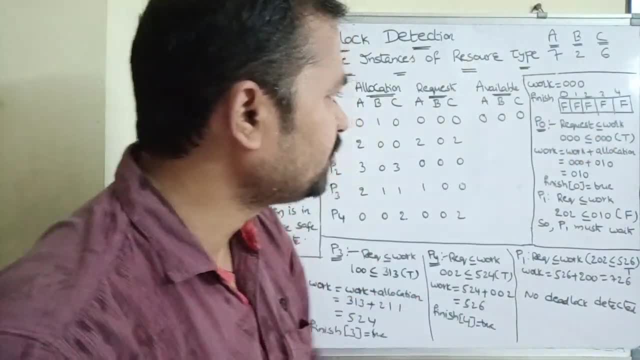 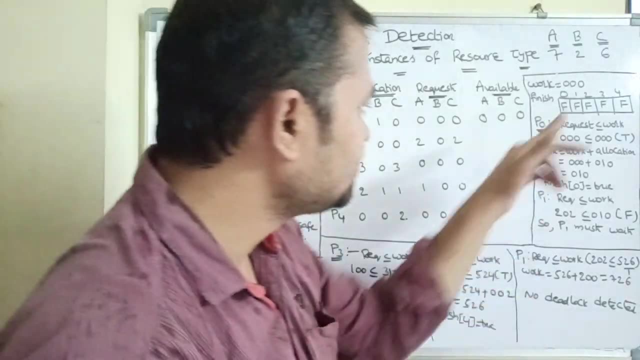 So work is equal to what are the available resources triple 0.. Next, for all the processes, allocation is not equal to 0. So finish of I is false. now, So finish of 0, f means false. 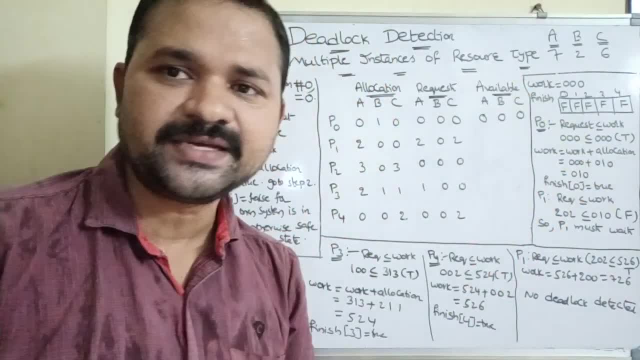 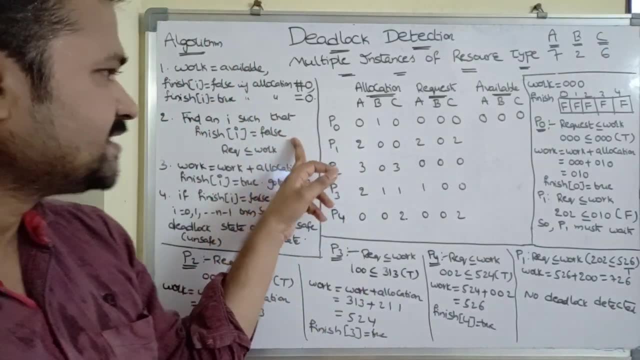 1 false, 2 false, 3 false, 4 false. So it specifies that the process execution is not completed till now. Let us see the second step. Find an I such that finish of I is false For all the processes. finish is false only. 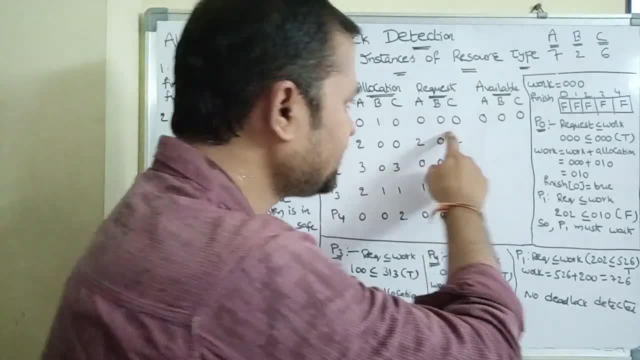 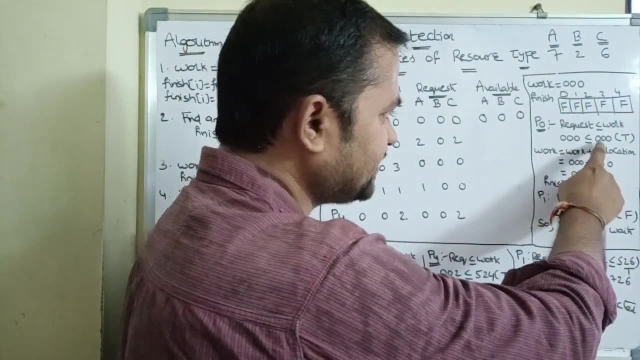 Request is less than or equal to work. So for P0, what is the request? Triple 0 is less than or equal to Work. means available. What is the work here? Triple 0.. So 0 is less than or equal to 0. 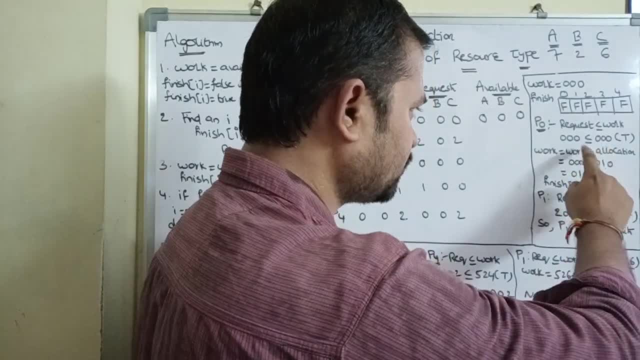 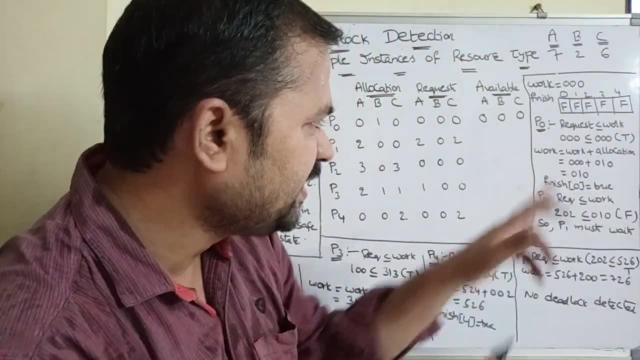 2. Next, B0 is less than or equal to B0.. Condition true: C0 is less than or equal to C. work Condition is true. So this condition is true, So we can complete P0 process execution now. 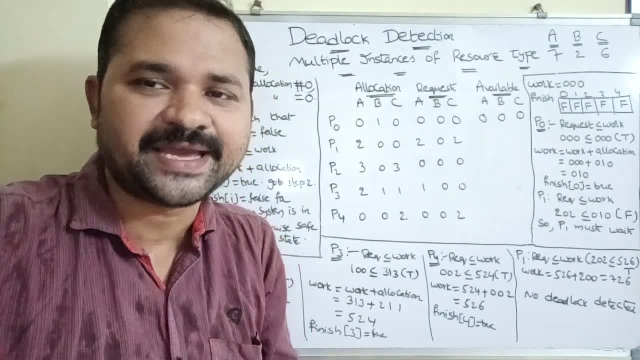 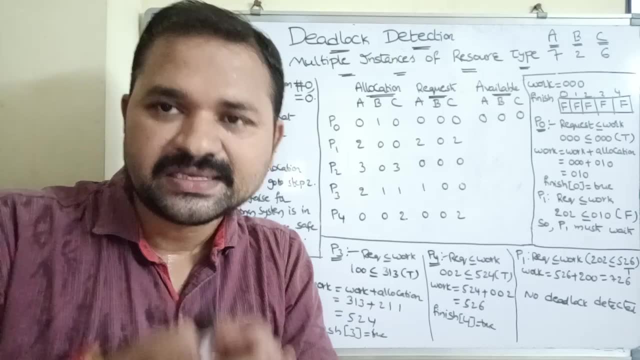 Why? Because request is less than or equal to work, So operating system can allocate the available resources to the work, So P0 can complete its execution. Once P0 execution is over, then the corresponding process is moved to the hard disk. 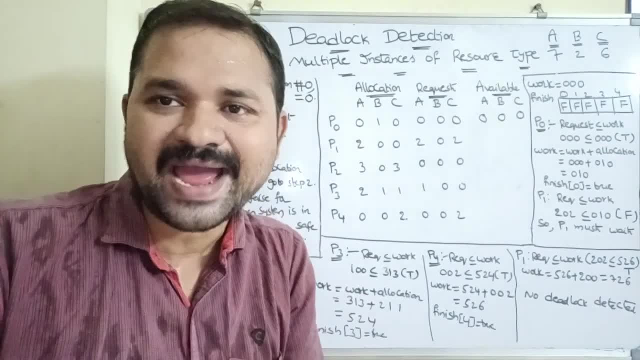 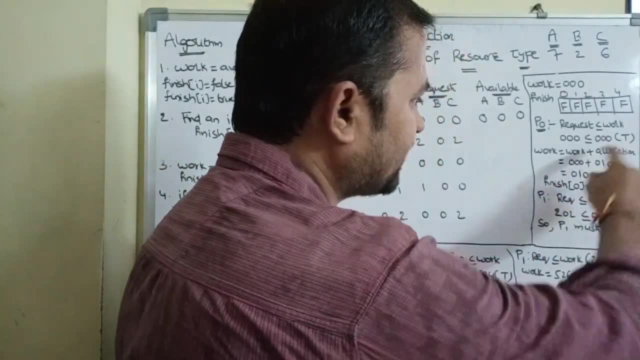 So we have to remove allocated resources of P0. And we add them to the work so that the available resources will become high. So work is equal to work plus allocation, So work value triple 0.. What are the allocated resources of P0?? 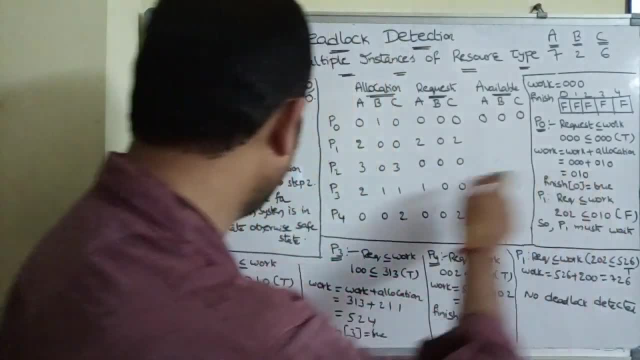 0, 1, 0.. So if we add them, then the result is 0, 1, 0.. So that is the third step here. Next, finish of I is equal to 2.. What is finish of I? 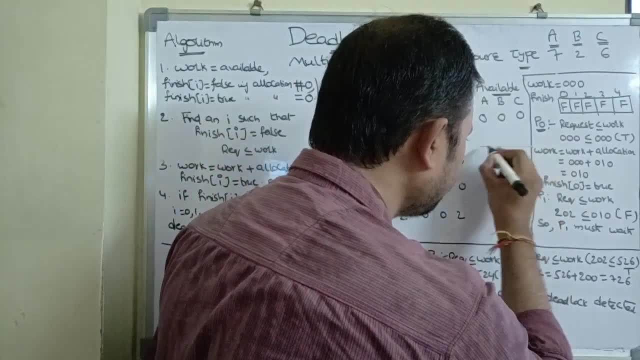 0.. So finish of 0 is equal to 2.. So that means here what is the first process we executed: P0.. So here this F is marked as 2, 0.. Okay, So that means here what is the first process we executed. 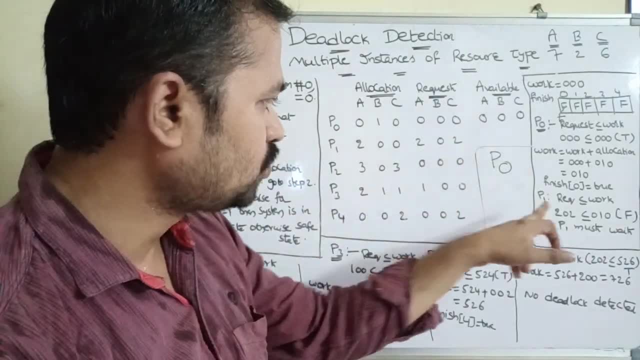 Next let us check for P1.. What is P1? request 2, 0, 2.. So 2, 0, 2 is less than or equal to What is the work here: 0, 1, 0.. 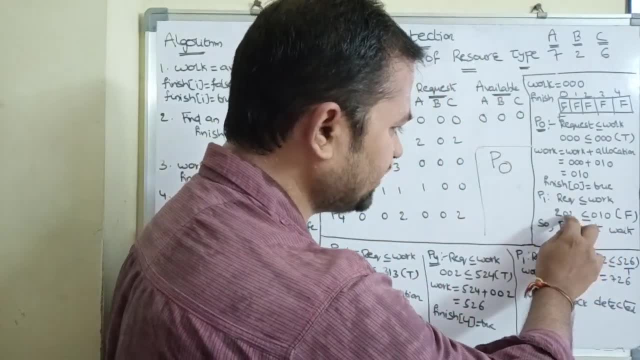 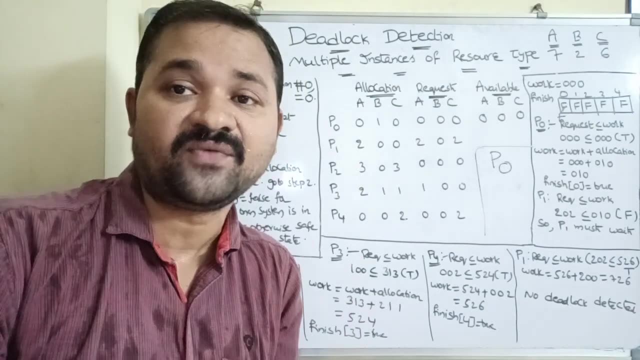 So 2 is less than 0. So this condition is false. So there is no need to check for B and C. So this condition is false. So P1 must wait until it gets sufficient number of resources for the operating system. 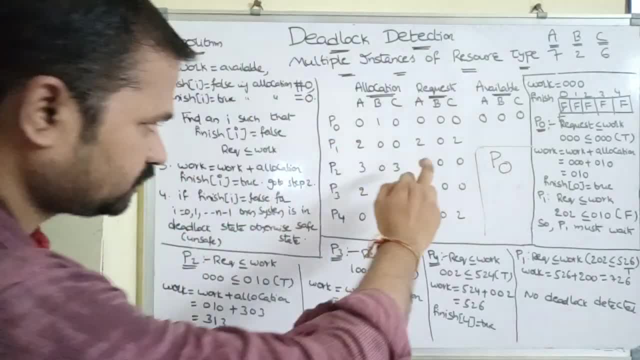 Now let us check for P2.. Request is less than or equal to work. What is P2 request? Triple 0.. Triple 0 is less than or equal to What is the work here? 0, 1, 0.. 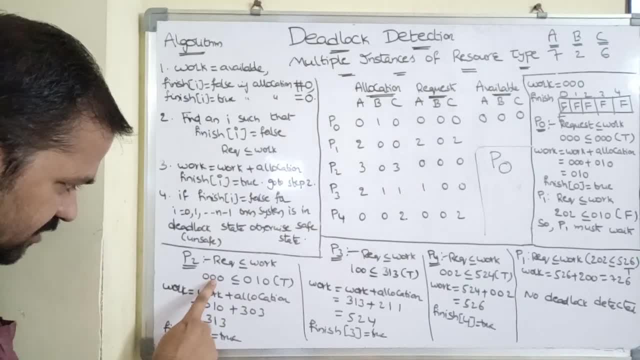 Yeah, 0 less than or equal to 0, 2.. Next, B: 0 less than or equal to 1,. 2.. C: 0 less than or equal to 0. Condition is true, So we can complete P2 execution now. 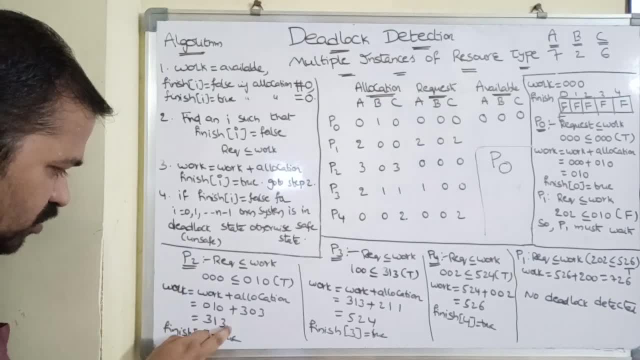 So operating system yards allocated resources of P2 to the work. Work means 0, 1, 0.. Next, what is P2 allocation resources? 3, 0.. If we add them then the result is 3, 1, 3.. 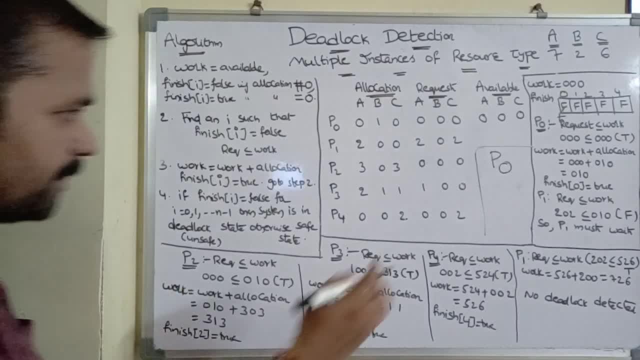 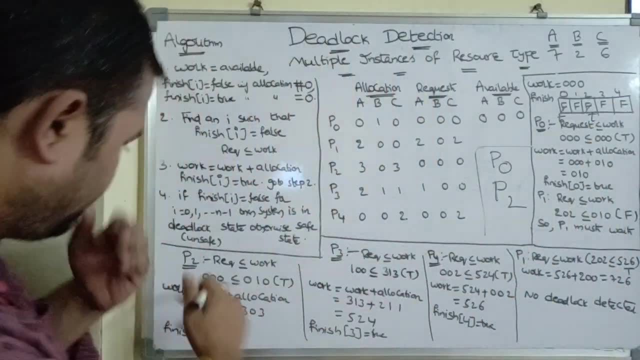 Next, finish of 2 is equal to 2.. So it specifies that P2 execution is over now. Okay, So we have to mark finish of 2 as true now. Okay, Next P2 is over. Now let us check for P3.. 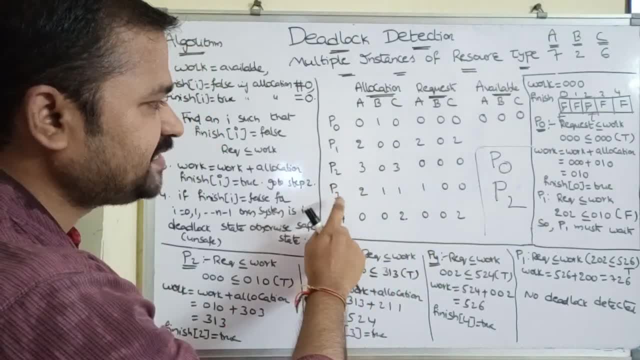 So what is P3 request? 1, 0, 0.. What is P3 work? Yeah, What are the available resources? 3, 1, 3.. So what is P3 request? 1, 0, 0.. 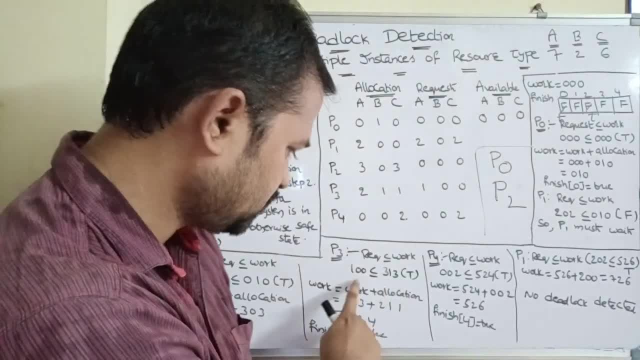 Next work: 3,, 1, 3.. So 1 less than or equal to 3.. So the first condition is false, For A also false, For A is false. So there is no need to check for P and C. 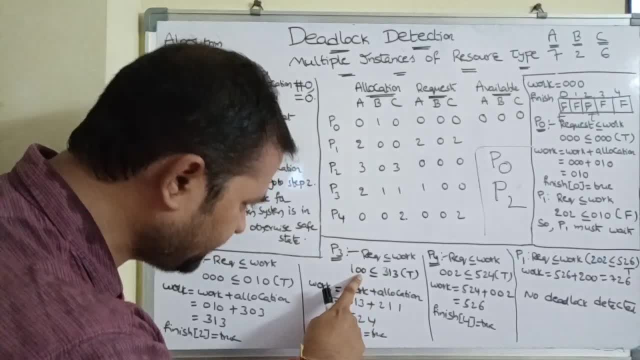 Yeah, I am sorry. 1 is less than or equal to 3.. True. Next, for resource type B: 0 is less than or equal to 1.. True 0 is less than or equal to 3.. 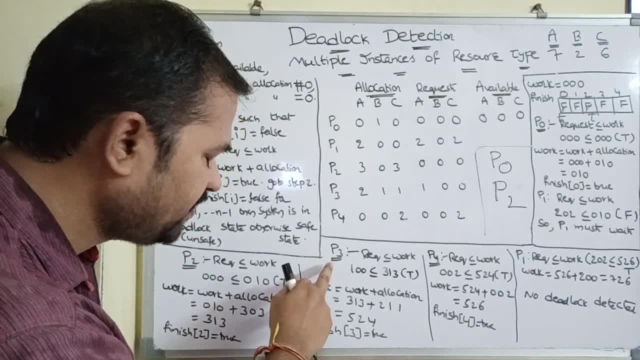 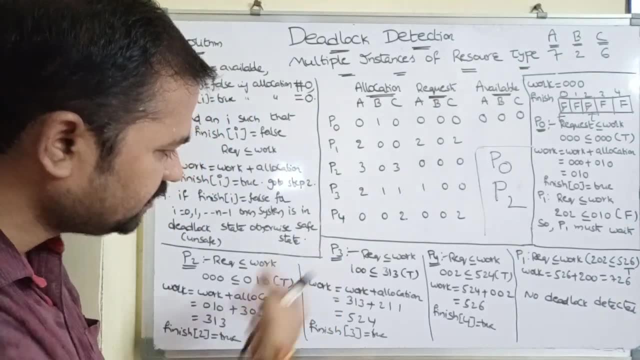 True. So here this condition is true, So we can complete P3 execution now. So once P3 execution is over, then add allocated resources of P3 to the work. So work is equal to work plus allocation. What is the work? 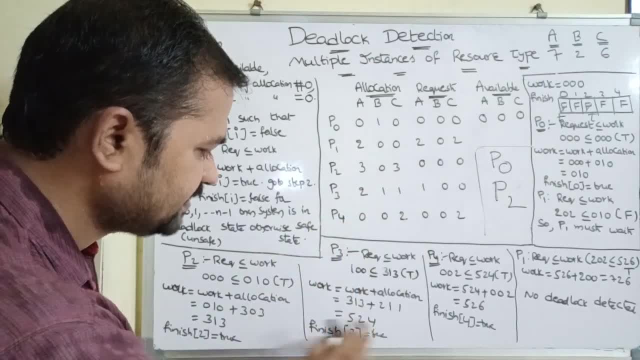 3, 1, 3.. What is P3? allocated resources: 2, double 1.. That is nothing but 5, 2, 4.. Finish of 3 is equal to true, So it specifies that P3 execution is over now. 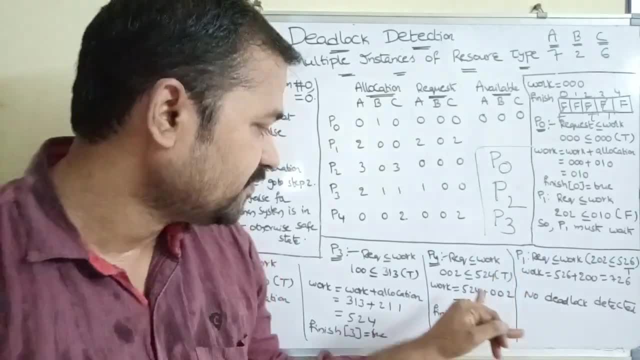 Now let us check for P4.. Request is less than or equal to work. What is P4 request 0, 0, 2.. So 0, 0, 2 is less than or equal to What is the work now? 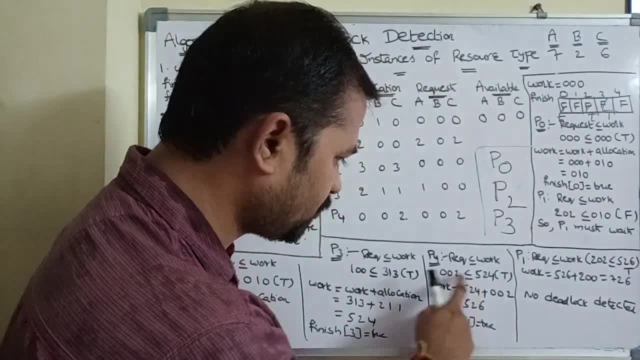 5,, 2,, 4.. So for resource type A: 0 less than or equal to 5.. True 0 less than or equal to 2.. True 2 less than or equal to 4.. 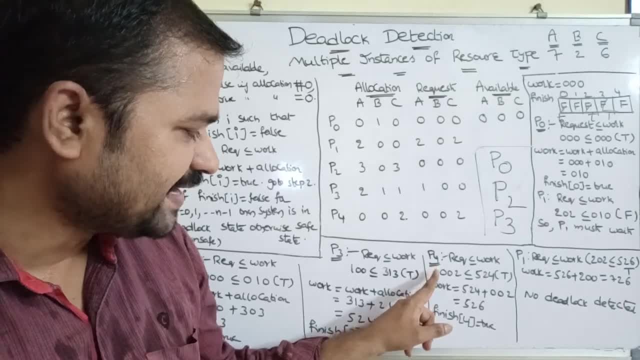 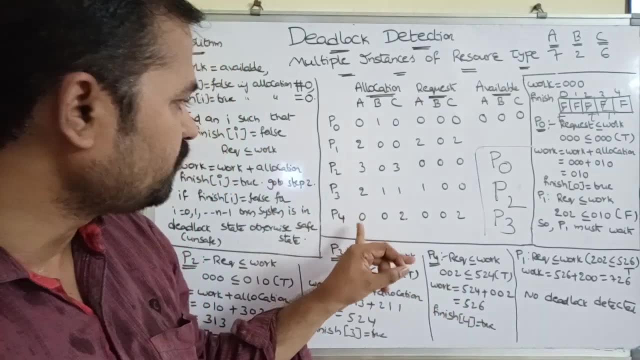 True, So we can complete P4 execution now. So we can add allocated resources of P4 to the work. So work is equal to what is the work: 5,, 2, 4.. Plus allocated resources of P4.. 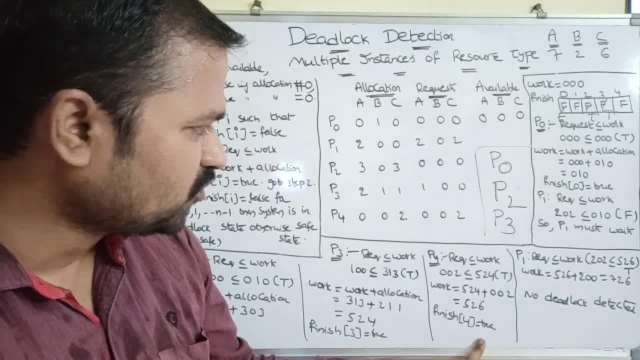 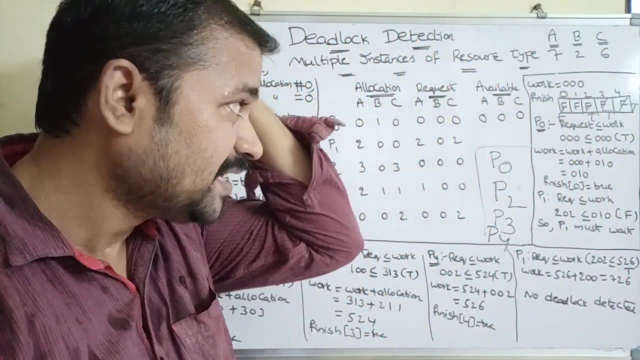 0, 0, 2.. That is nothing but 5,, 2, 6.. So finish of 4 is equal to 2.. So that means P4 execution is over now. Now we have to come from the first process and check whether there is any process which 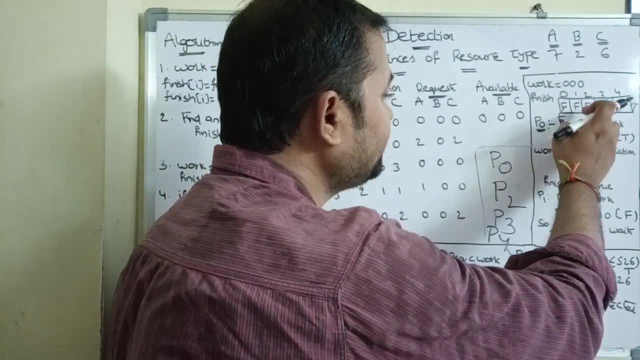 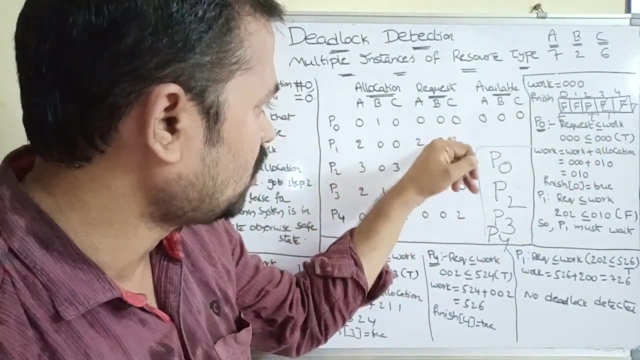 is not executed or not. So finish of 0 is already executed, But finish of 1 is not executed. Process 1 is not executed. So let us take P1 request now 2, 0, 2.. 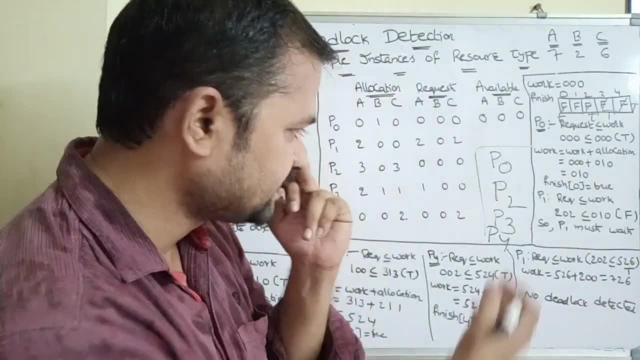 So 2, 0, 2 is less than or equal to work. What is the work here? 5, 2, 6.. Condition is true, So we can execute P1 process now. So after execution we can add: 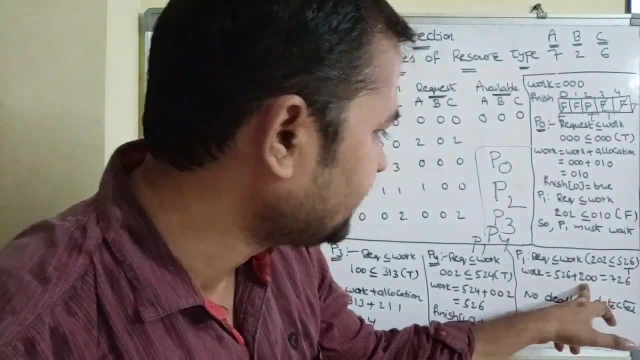 Allocated resources of P1 to the work. So work is equal to work plus allocation. What is work? 5, 2, 6.. Plus P1 allocated resources: 2, 0, 0. That is nothing but 7, 2, 6.. 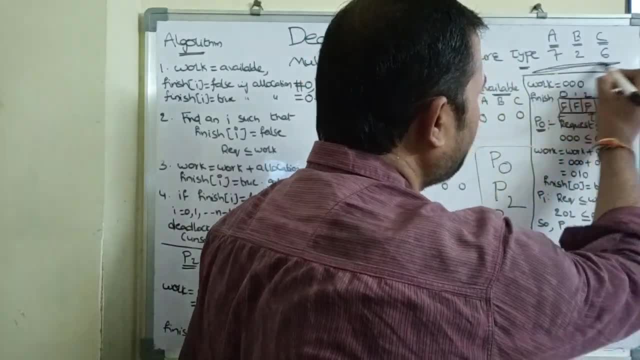 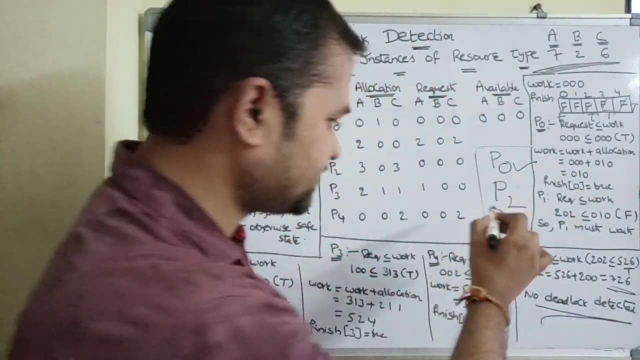 Here this 7, 2, 6, is nothing but the initial number of available resources. Okay, So here we can say that there is no deadlock is detected, So P0.. This is the same sequence, So P0, P2, P3, P4.